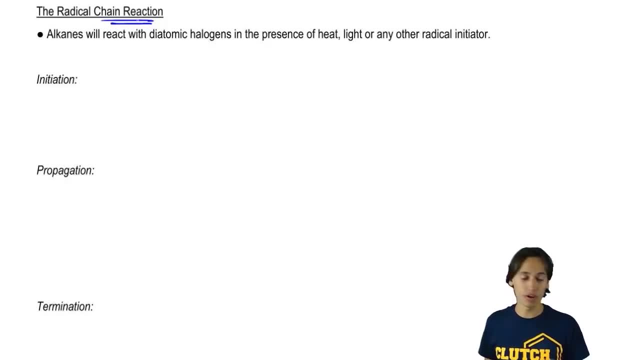 and we're actually going to need to write all three of these steps. In fact, it's smart that you actually write the words. if you do have to draw this mechanism for a test, that you write these three words: initiation, propagation and termination. 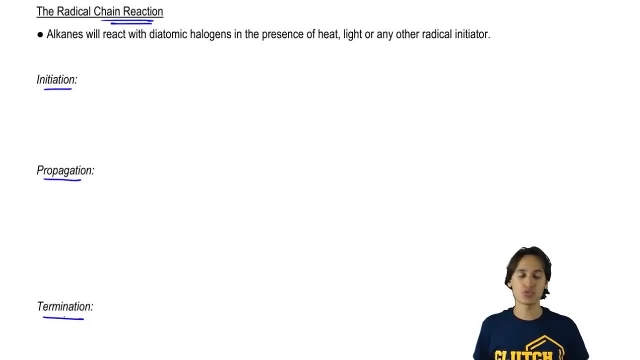 So let's look at the initiation step And let's say that we're just using the easiest radical initiator, which is X2.. And let's use X2 over heat. Okay, Now, what I taught you guys is that, in the initiation step, what we're going to wind, 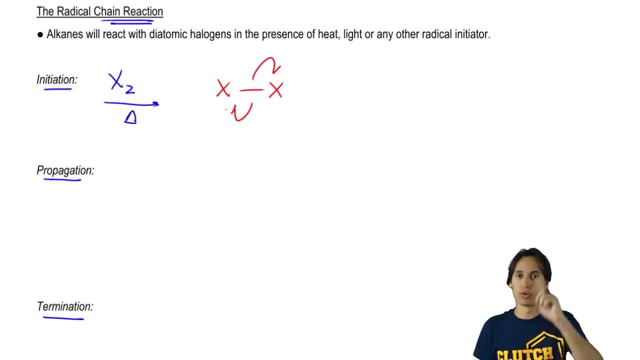 up getting is electrons from two electrons, one on each side, jumping onto each X. So what I'm going to wind up getting is X radical plus X radical. That's the end of my initiation step. Really, all I need for the bare minimum of my initiation step to work, all I need is 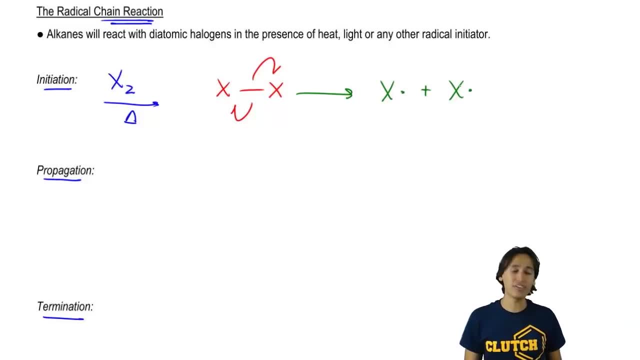 one radical. In this case I have two, So I'm great. Okay, So now that I have that radical in place, that radical is free to react with other molecules, And it turns out that it happens to react really well with alkanes. 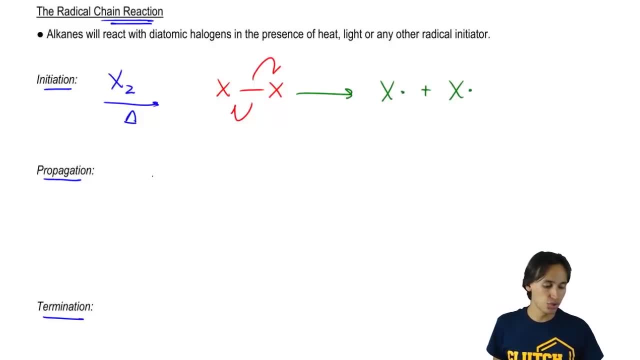 Now, for the sake of a really simple mechanism, let's just use the simplest alkane possible, which is methane, methane just being a one-carbon hydrocarbon, CH4.. So now I've got CH4 and I'm reacting that with X radical. 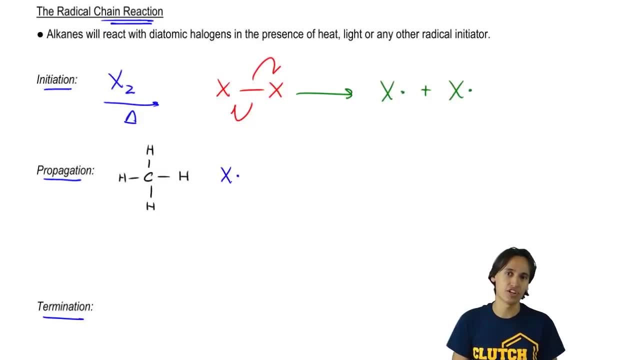 Okay. So this X radical hates itself. right now It's super high energy, super unstable. It's saying: how can I get rid of this hot potato, How can I get rid of it? And then it sees all these electrons in the methane and it's thinking, hmm, maybe I can. 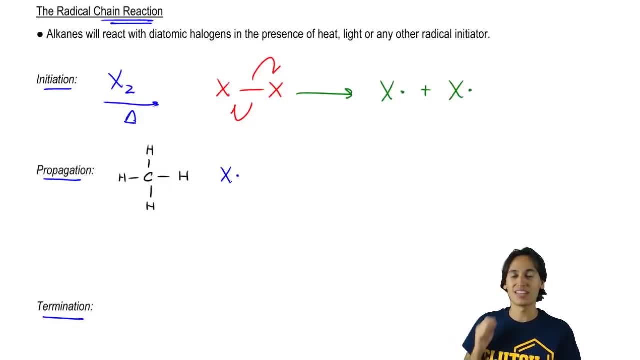 take one of the electrons from one of those carbon-hydrogen bonds, And that's exactly what it does. So it turns out that radicals are going to react with hydrogens in alkanes, And the way we draw these arrows is just so. you know, radical reactions are always going. 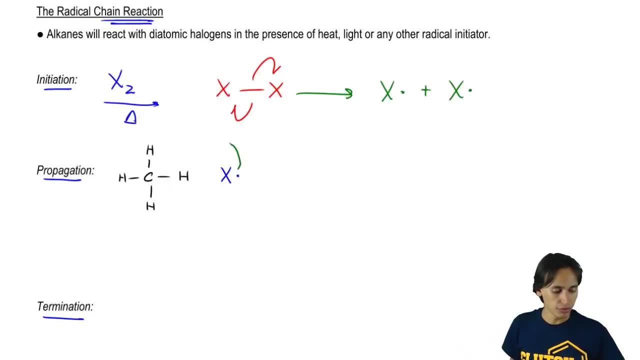 to have three arrows. So I'm going to draw one fish hook into the middle of nowhere. Then I'm going to draw another fish hook from the CH bond meeting that one. What that's implying is that now there's going to be a new bond between the H and the X. that's 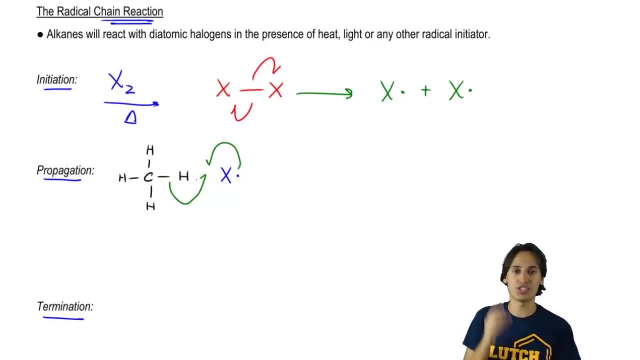 going to form from those two electrons. So that's looking great, but I still have one electron left over. Notice that the bond between the CH had two electrons. So where do you think that last electron goes? It goes onto the C, Okay. 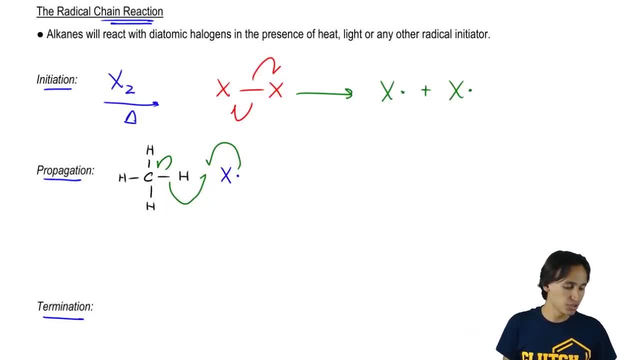 It goes on. It goes onto the carbon backbone. So what that's going to do is it's going to give me a structure that now looks like this: C, H, H, H, radical. Now notice that I'm drawing the geometry different, because now this would be trigonal planar. 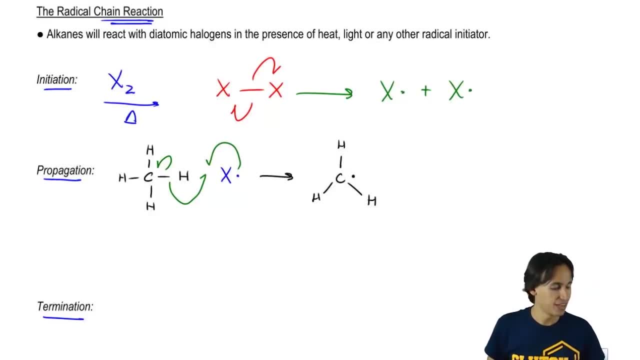 So you should draw it like a triangle and that would be plus HX Making sense so far. So notice that the reason this is called a propagation step is because propagation means I'm reproducing, myself propagating, And notice that the radical just reproduced itself. 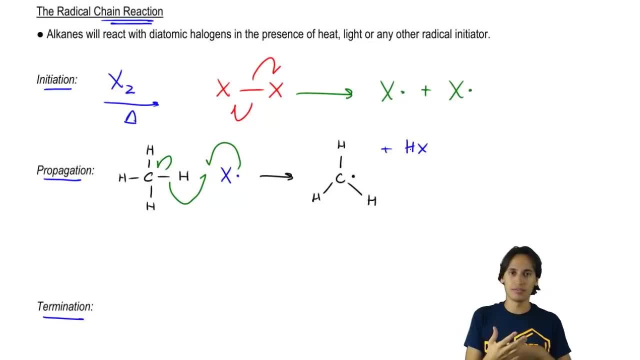 Now it kind of moved through my medium and now I've got a radical on a new species. Well, it turns out that your propagation step isn't done yet, because you're not done with the propagation step until you fully reproduce yourself 100%. So what that means is: not only do I need to have a radical at the end, I need to have 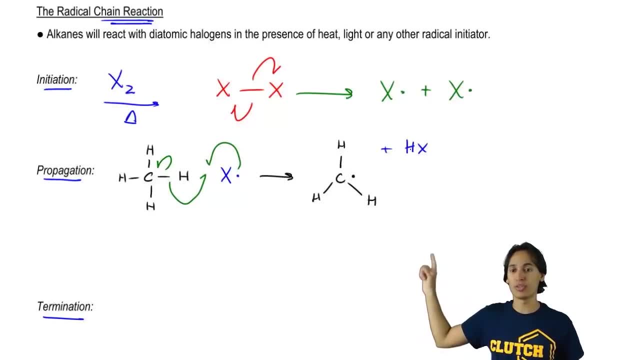 the same exact radical that I started with. So if I start off with an X radical, I need to end off with an X radical. So what that means is what could I? – we're actually just in the middle of our propagation step right now. 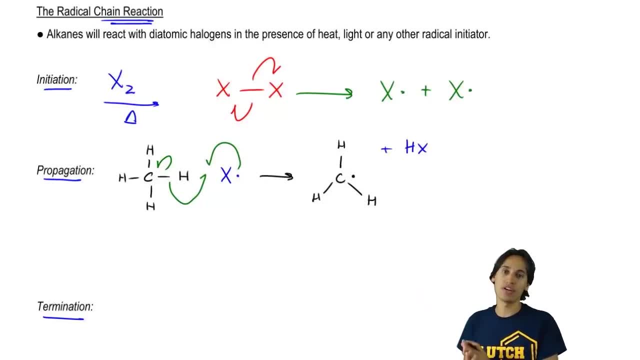 What could we react my C radical with to generate that original X radical that we had at the beginning? Can you think of anything It turns out? the easiest thing to do is just to react it with another X, X diatomic halogen. 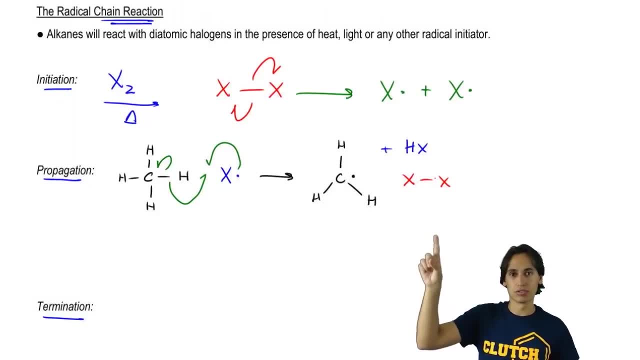 Now you might be wondering: Well, Johnny, why isn't this already radical? Because we just did that in the first step. We made it radical. Well, it turns out that not all of the diatomic halogen is going to cleave at the same time. 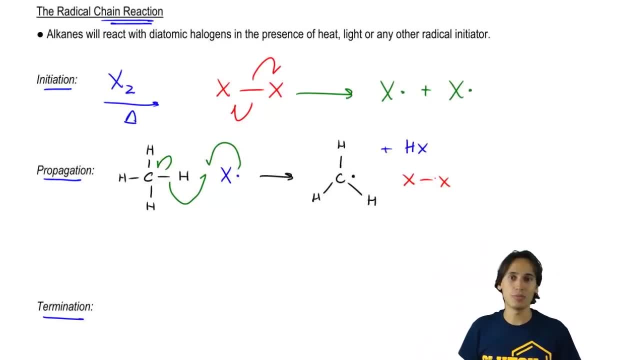 So some of it's going to do the initiation step, but some of it isn't going to be hit by enough light or enough heat to split up yet. So what that means is that the one I'm reacting with here hasn't cleaved yet. 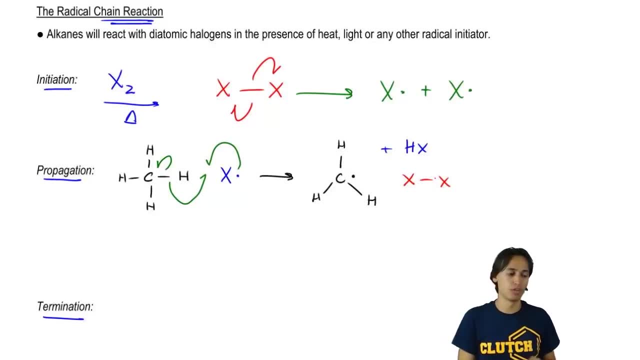 So this is one that's just waiting around for enough energy to finally do that homolytic cleavage Before the light can even get to it. another radical just did So. instead, we're going to propagate to the X- X, And the way we draw these arrows is once again, three arrows. 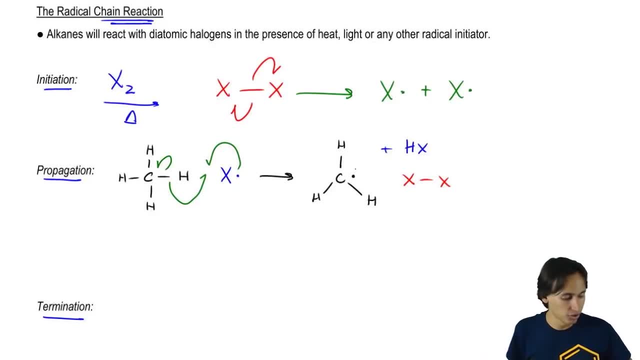 So I'm going to take – the radical always starts it. I'm going to take the radical. I'm going to put that one out into the middle of nowhere between the C and the X. So then I'm going to take one electron from this bond and make it go there. 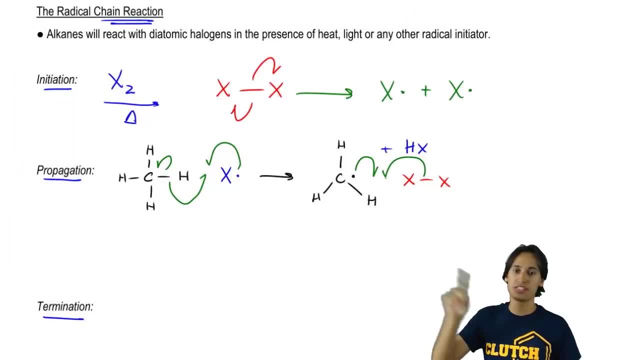 This represents that now there's going to be a new bond of two electrons between the C and the X, But unfortunately I've got one electron left. All right, So that's left over. I'm going to dump that one onto the X. 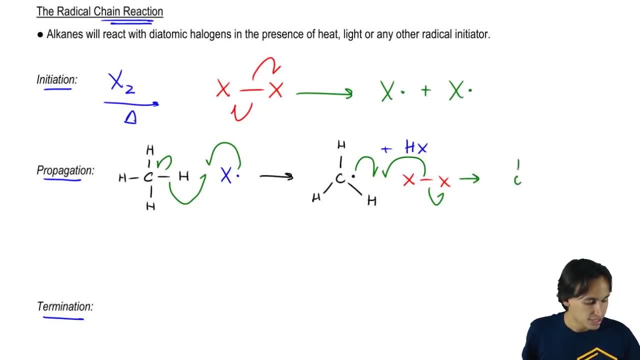 So what I'm going to get at the end of this step is now notice C, H, H, H. but now I've got an X. What do we call that functional group when you have a carbon and a halogen attached to each other? 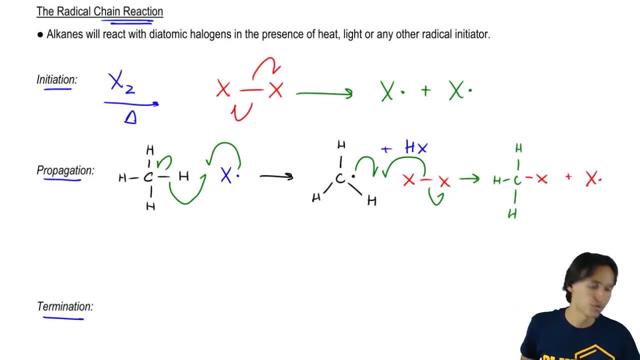 Alkyl halide And notice that now I'm going to have X radical. So that's the end of my propagation step, because now I have the same exact radical that I started with And notice that my propagation step just created a very useful byproduct, which is that it. 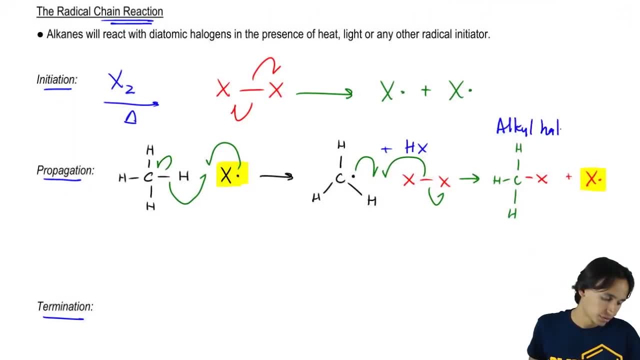 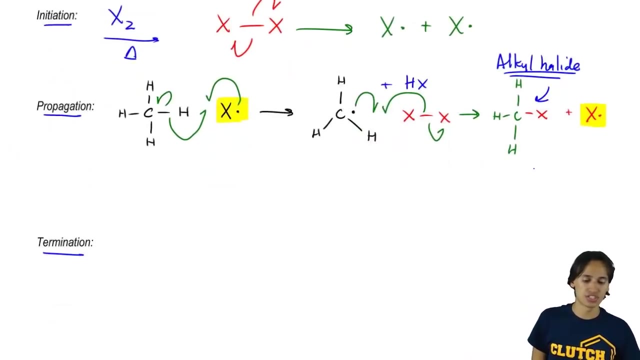 made an alkyl halide which, like I said, alkyl halides do a whole lot more stuff than alkanes do, So this is a very useful reaction for me as an organic chemist. So now we're going to do our termination step. 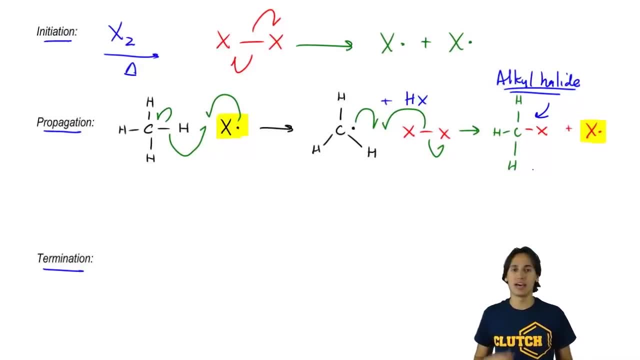 Now, what is termination? Termination means that you're producing all these radicals. These radicals are spreading Radical, radical, radical. You're generating all of them. What happens in termination is that you finally have so many radicals that, instead of propagating, 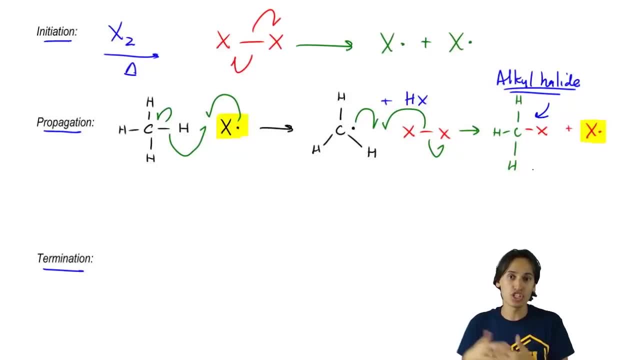 and forming new radicals. they're actually extinguishing each other faster than they can make new radicals. Because, think about it: If you have two radicals coming together, if they hit each other, what do you think is going to happen? Well, I've got one electron here, one electron here. 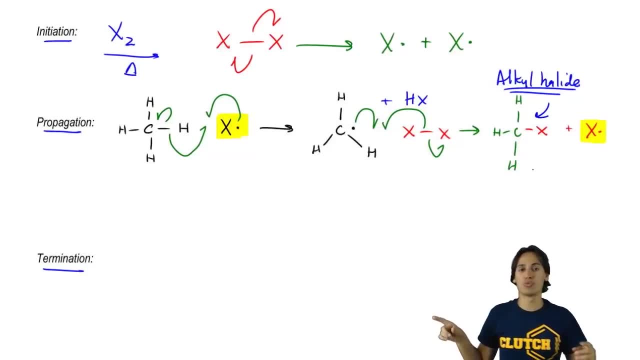 They're going to form a new bond. So the termination phase is what happens when there's so many radicals that they actually bump into each other. They collide into each other more often than they collide into unreacted species. So in my termination phase what I do is I look at all the different possibilities of 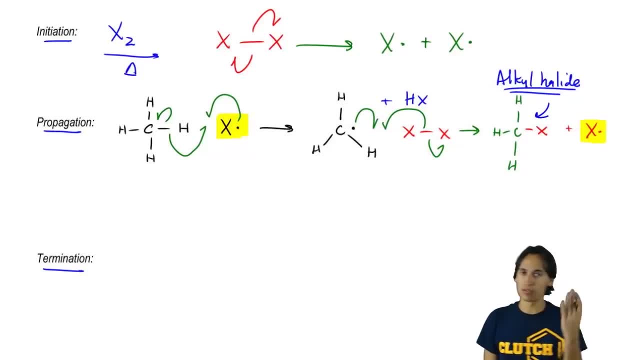 radicals that could have collided. So the easiest radicals to think of that could have collided are the radicals that collide, The radicals that collide. The radicals that collide, could have collided are just X plus X, because these were being formed in high amounts. What happens if they hit each other? 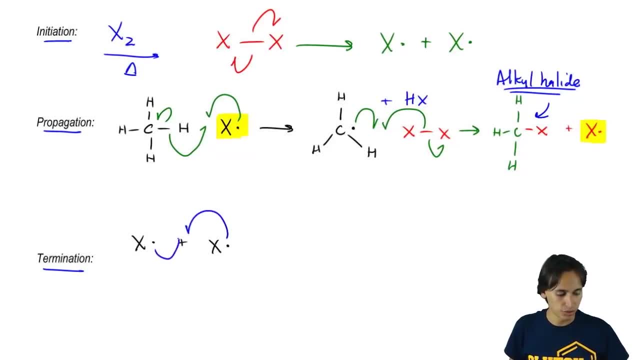 Well, I would just wind up getting the same thing all over again. I would do this, I would do that And I would get XX. So that's one termination product, But there are actually some other termination products possible. Can you think of another one? 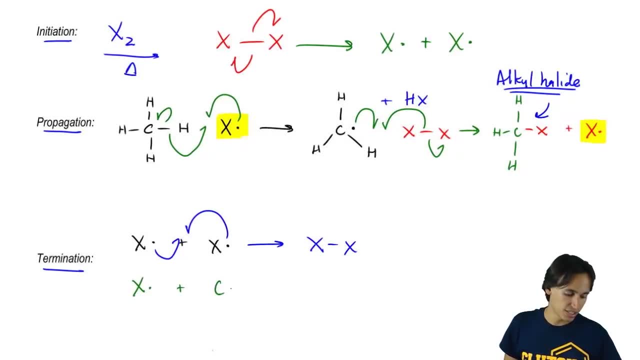 Another one would be if I had an X radical and a C radical. Okay, That would be like the radical that I had up here in black, where maybe, instead of hitting an XX that wasn't reacted yet, maybe it reacts with a radical. Once again, I get my arrows. 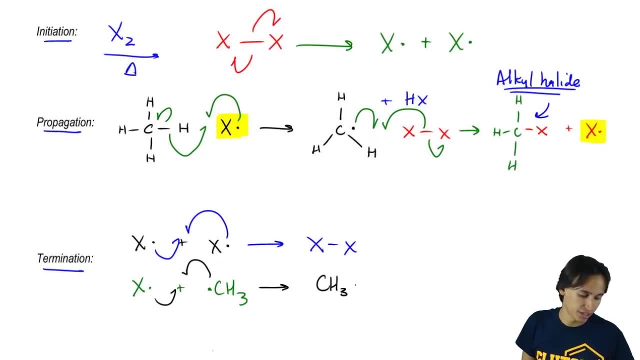 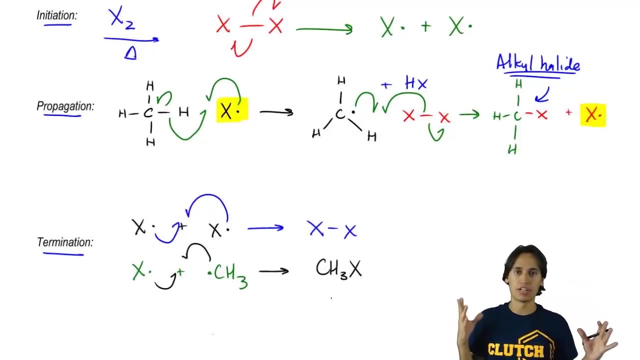 And what I get as a product here would be CH3X, So I get an alkyl halide. Can you guys think of any more combinations? There actually is one more, And that last one would be what? What if I got CH3 radical plus CH3 radical? 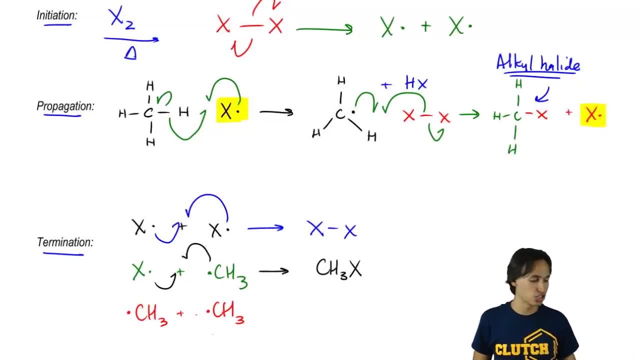 Now this is tricky because now it looks like I'm going to get a completely different product, And it's true. What I would get now is actually ethane, CH3CH3.. Crazy, right. So now, what I just did is I just made a larger hydrocarbon than before. 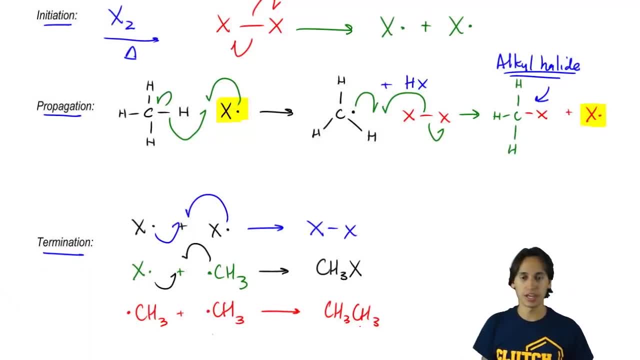 Before I just started off with methane and now I'm getting ethane as a product. Well, a few notes about these termination products. First of all, the first one is not going to really matter, So I'm just going to say: I don't know. I'm trying to think of a symbol that I can use. 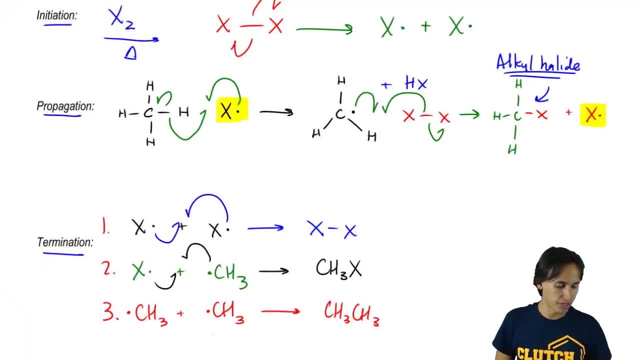 But just like, let's say, I have termination product 1,, 2, and 3, right. Number 1 isn't really going to matter that much, And the reason is because after I make the X2, it can then just react with heat or light. 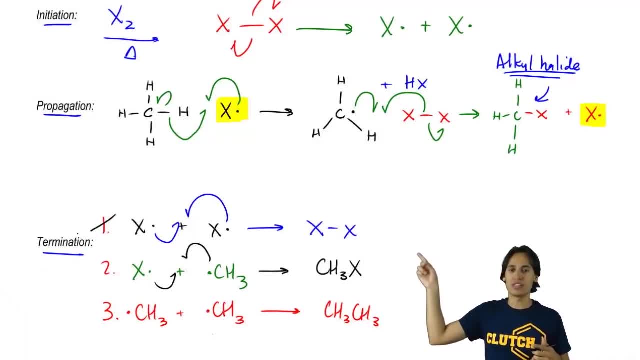 again and make radicals again. So really this is a termination phase. that happens And then it disappears. And then it disappears Okay, And then it disassociates again. So you're not going to get a whole lot of X2 forming because the X2 keeps breaking up. 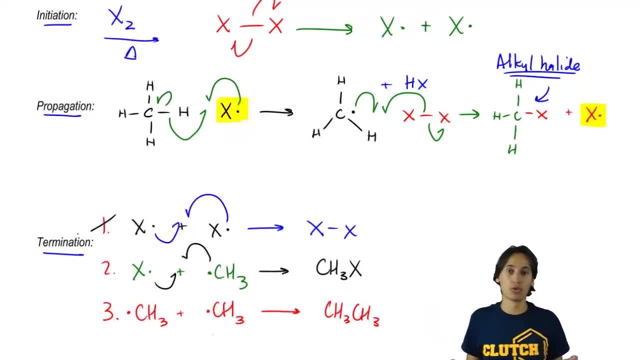 Okay, So that's the first thing. So actually, X2 isn't going to form a whole lot Now. your professor still probably wants to see that termination step, But just as your final product, you're not going to get a whole lot of X2 as a final. 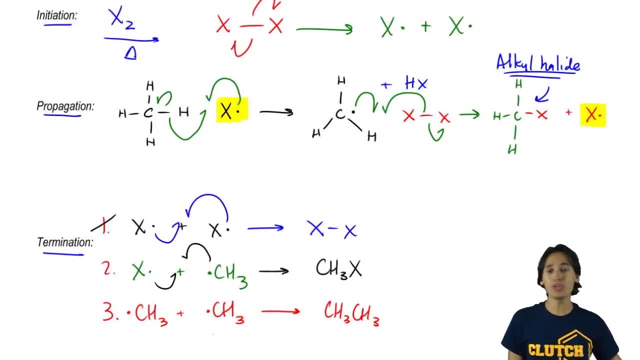 product. Okay, So you can cancel out 1.. Another one that we can cancel out is actually 3.. The reason is because the only way that I can form ethane here is if I have a CH3, a methyl-radical and a methyl-radical colliding. 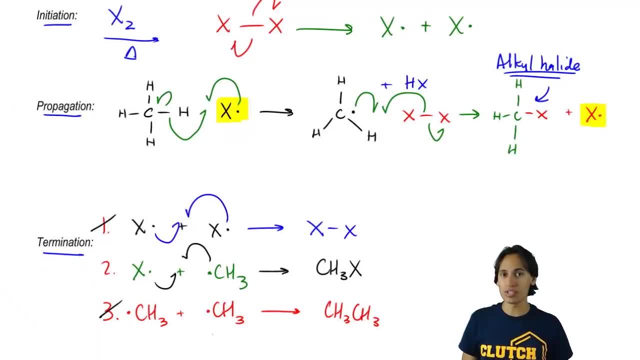 Well, the chances of having methyl-radicals is actually way lower than the chances of having a halogen radical. Why? Because you're forming the halogen radicals directly through my energy, through my light or my heat, Whereas these methyl-radicals can only be formed after they've already reacted with. 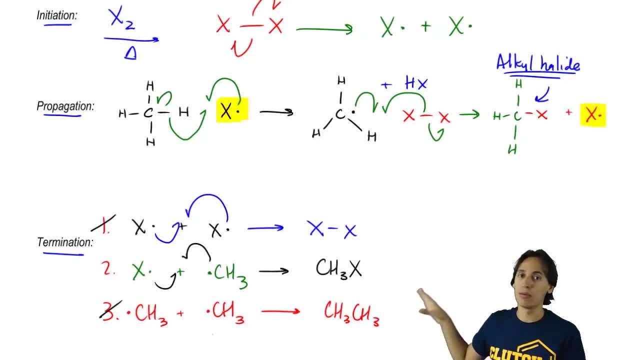 a halogen, So the chances of them colliding and making a bigger hydrocarbon are actually very small compared to the chances of them colliding And with another halogen. So what I would say is that I'm going to get a very tiny amount of this like scarce. 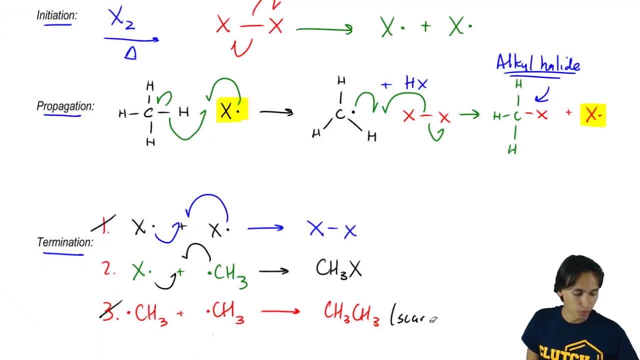 Let me try that one more time: Scarce- Wow, I'm really bad at spelling, guys. Sorry, Scarce. I would get a tiny amount of this, but it's not going to be a huge amount. It turns out that there's actually a way that we can even lower this even more. 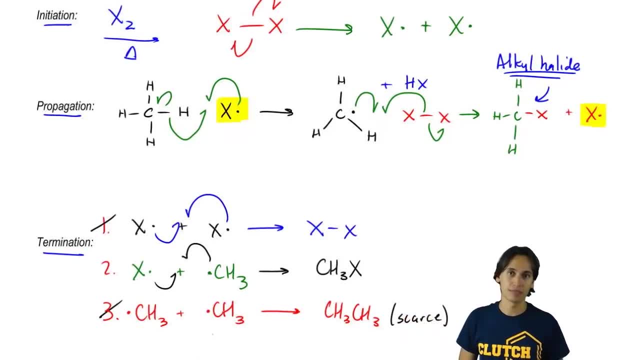 We could lower the amount of my larger alkanes that we have, And the way we could do that is just by reacting with excess halogen. If I just react with a lot of halogen and a very low quantity of alkane, then that even 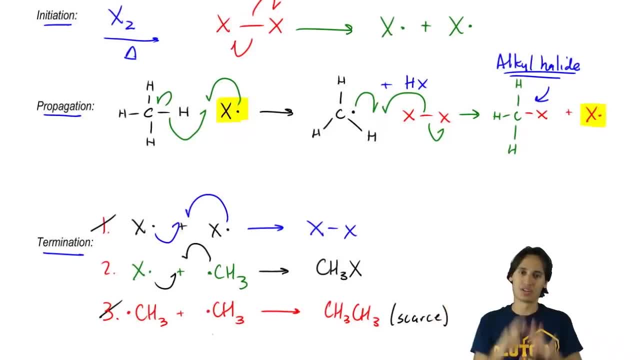 reduces the chances more that two alkane radicals are going to collide. So, depending on what my concentration is of alkane, I could basically take this down to zero. If I really wanted to, I could take this down to pretty much full zero. 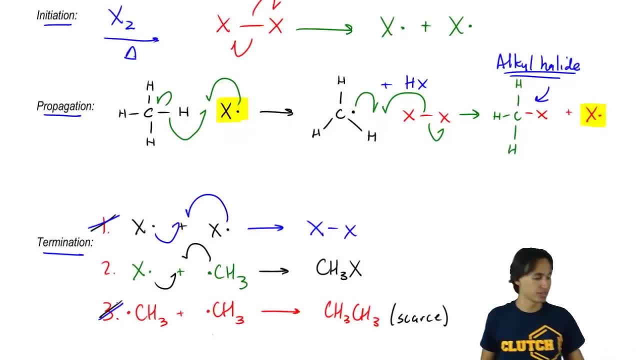 So we're going to cross out one and three. That means that what's my real main product? Well, the real product is going to be my alkyl halide, And that's the whole point of these. Let me just move out of the way.